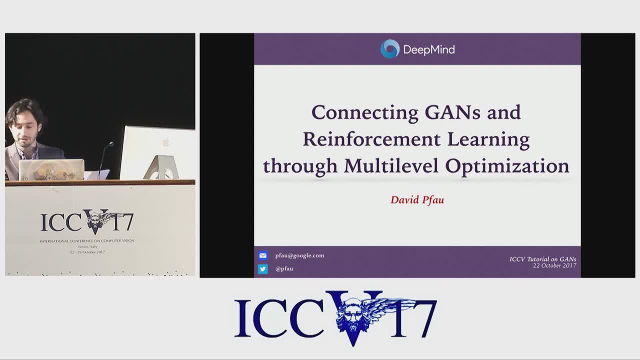 All right, Thank you, Ian, and thank you all for coming. So I'm going to talk about these connections between generative adversarial networks and reinforcement learning, largely through the lens of optimization. There's a very surprisingly close connection between models in what seems like should be very disparate fields in machine learning, And many of the problems we face at DeepMind training. reinforcement learning models are very similar to the issues faced when training GANs. 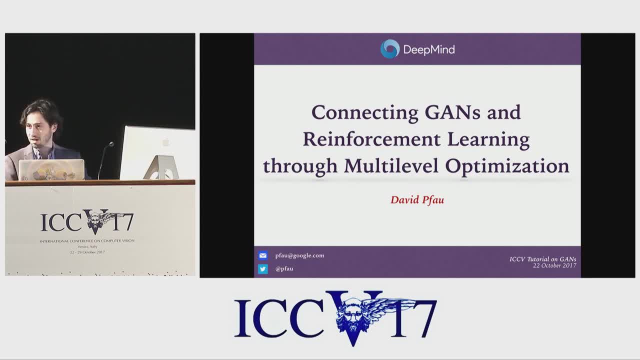 And I think that this is a underappreciated connection. A lot of the heuristics that are developed in one field can be transferred to the other, And there's a lot of room for a rich, rich interplay between the two. 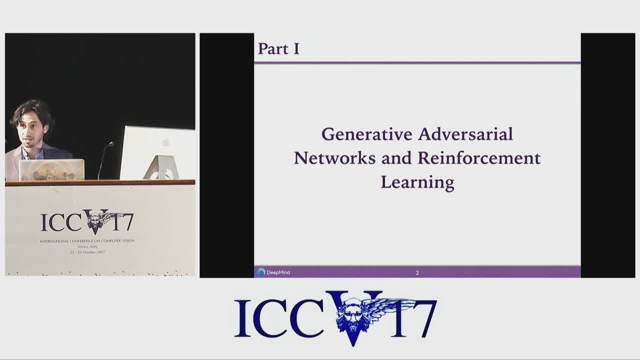 So, just to start, I want to explain what the major similarities are between GANs and many RL algorithms. The short answer is that they're both instances of what's called multi-level optimization, And understanding that, I think, is really the central idea in understanding how to better train GANs. 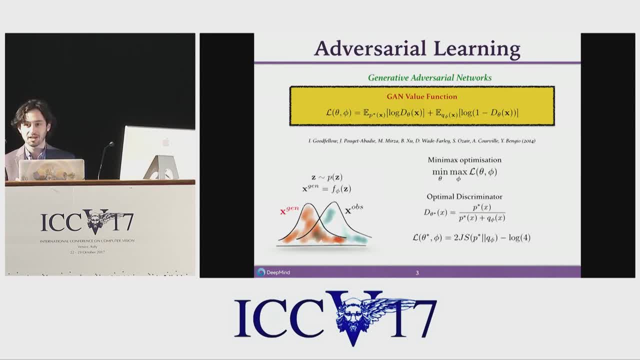 So for the those of you who've been here for the other talks, this should already be quite familiar. But just one more time: generative adversarial networks are trying to optimize not a loss function but a value function. So rather than being a direct minimization problem, it's a minimax problem. 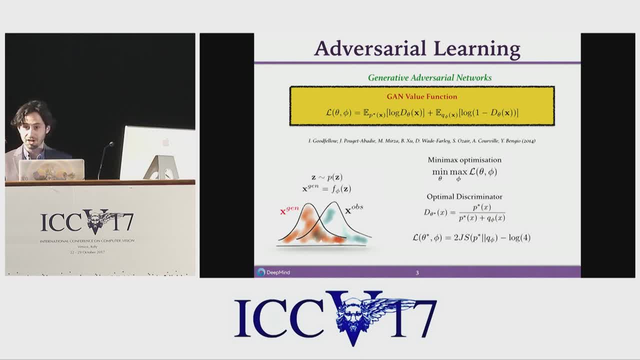 So you have a discriminator that's trying to minimize this loss and a generator that's trying to maximize it. In the case where you can compute the exact density for your generator, you can write down the optimal discriminator and close down the right-hand side. 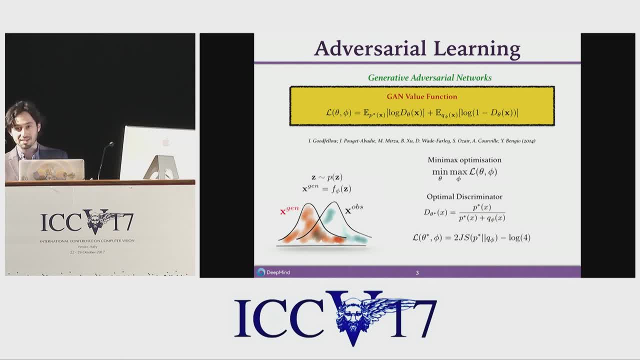 discriminator in closed form, and then this becomes equivalent to minimizing a Jensen-Shannon divergence between generated and real distributions. There are other formulations of the GAN problem that minimize other distances, like the Wasserstein loss, but in practice the motivation behind GANs is really that you should be able to greatly expand the class of generative models. 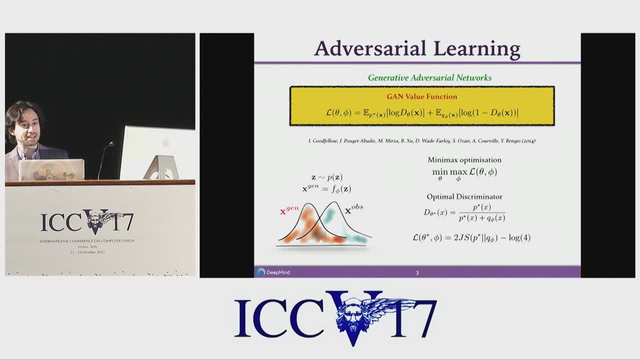 you can look at if you give up trying to exactly compute a density and instead approximate this discriminator with a neural network and also train it with gradient descent. So we want to look at other cases in the machine learning model where these kinds of optimization problems appear In practice. typically you 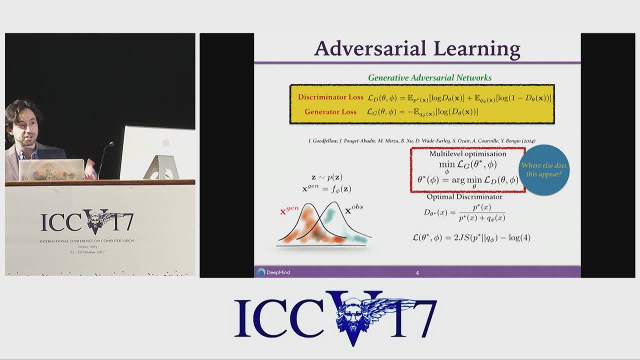 actually use the slightly tighter vorne somewhat more traditionally in this progression of slightly different loss for the generator, which is the difference between trying to maximize the misclassification rate or minimize the classification rate. This leads to improvements in the gradients when you're far away from a solution. 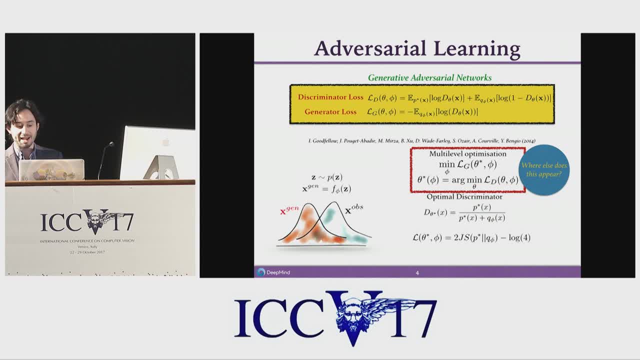 And that actually means that you're no longer strictly solving a minimax problem. you're actually solving a more general kind of optimization problem called a bi-level or multi-level optimization problem, And in its most general formulation, a bi-level problem looks like this: 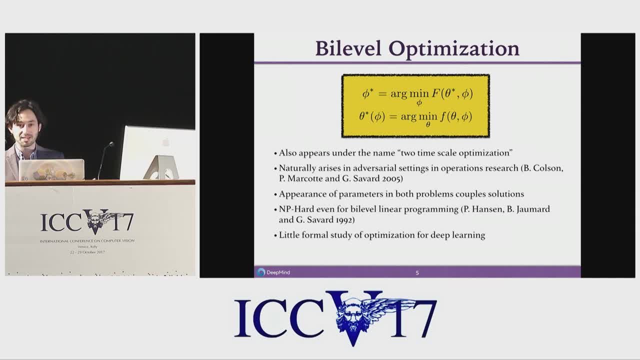 This is also sometimes referred to as two timescale optimizations, because it's really two nested optimization problems. You have one high-level optimization problem where one of the terms in it- this theta term, is itself the solution to another lower-level optimization problem And the reason you can't just sort of trivially solve this. 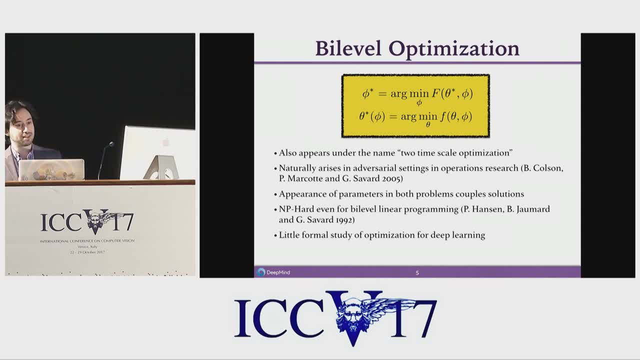 optimization problem yourself, like any other optimization problem, is that the inner loss function depends on the parameters of the outer loss function. So anytime you make an update to the outer loss function, this theta star solution to the inner function actually changes, And this introduces coupling between the two models. that makes this a significantly harder. 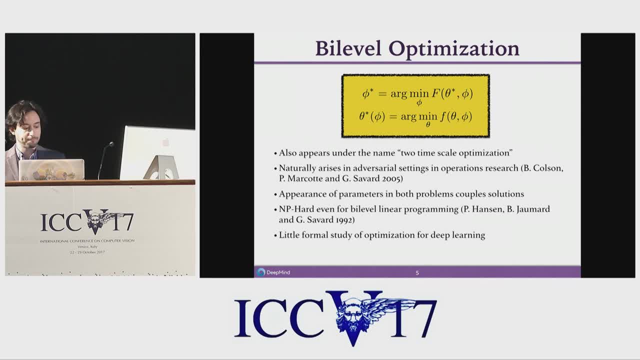 problem than just single-level optimization. So this comes up all the time in operations research. If, for instance, you're looking at a single-level optimization, you're going to have all of these problems, So you're gonna have to do an optimization of each one. 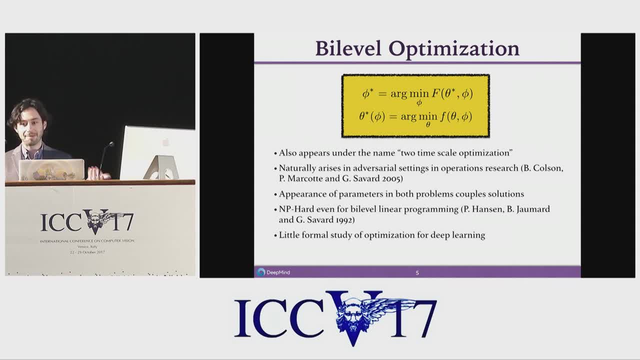 instance, you have a high-level problem, that's maybe a firm trying to maximize its profits, and a low-level problem that's a model of an individual consumer trying to decide between different firms. So a lot of formal theory has gone into studying this. typically, in the case where both the 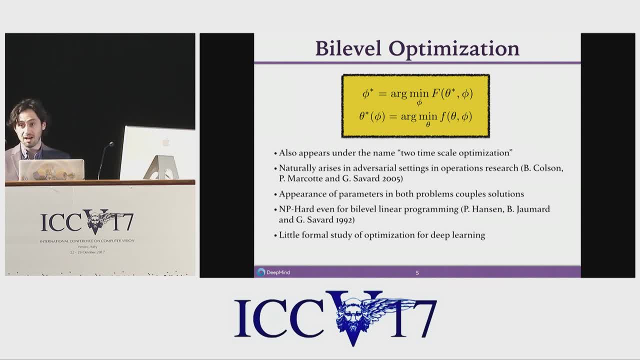 outer and inner problems are instances of, say, linear programs, and in that case it's been proven that this is an NP-hard problem, even though a single-level linear programming problem is much easier. it just can be solved in polynomial time. So even introducing this one extra layer suddenly takes you from something that's solvable to 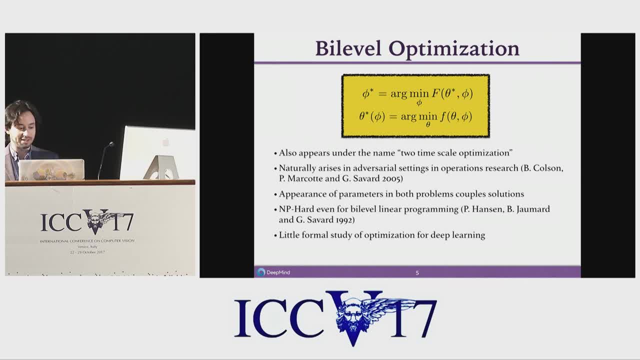 something where often the hope of an exact solution goes out the window. But in the case of deep learning you don't really care about exactly solving these problems, you just want to get a good local saddle point, And I think there hasn't really been much formal study. 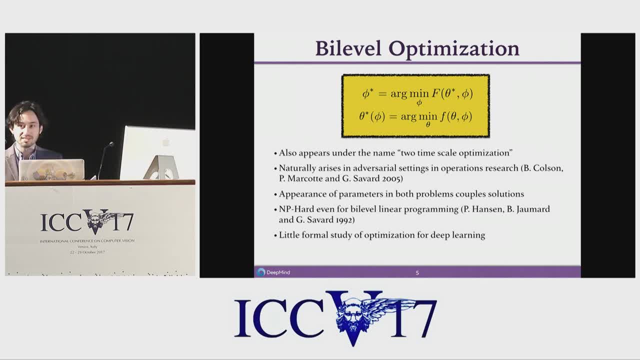 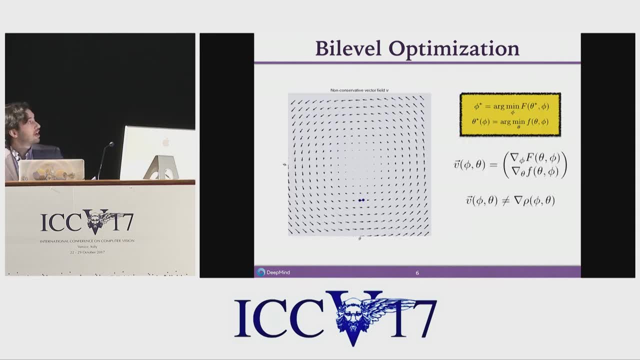 So the sort of simplest illustration of the kind of problems that you get from this coupling generally looks something like this: This is a figure. thanks to Frank Hushar for this. This is just an example of a minimax problem trying to solve the value where the value. 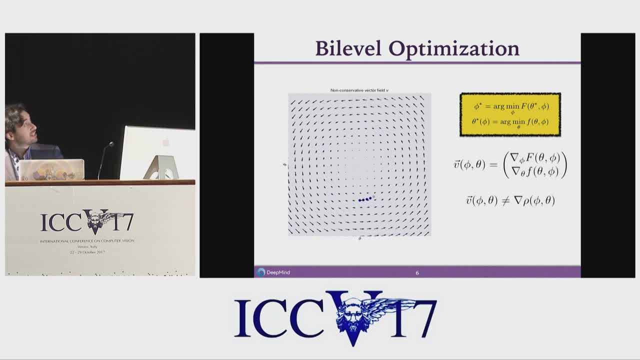 function is just theta times the value of the value function. There's a nonlinear expression for this. This is theta times phi And the gradients look like this vector field with a large curl. Clearly, if you just try to solve this by alternating or simultaneously doing gradient. 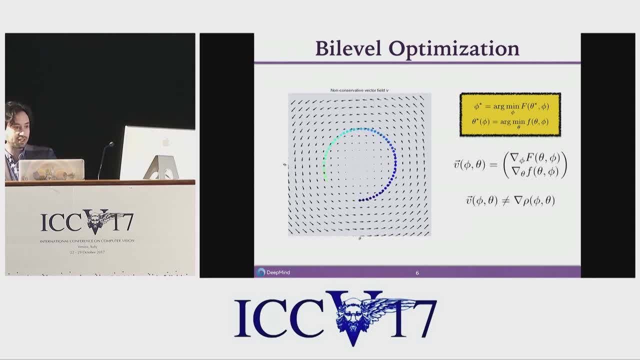 descent. you'll just sort of oscillate endlessly, And this is because there's no scalar function that has gradients that give you this gradient field. So this is a strictly larger class of problems than just single-level optimization. Ends No 9: 0. 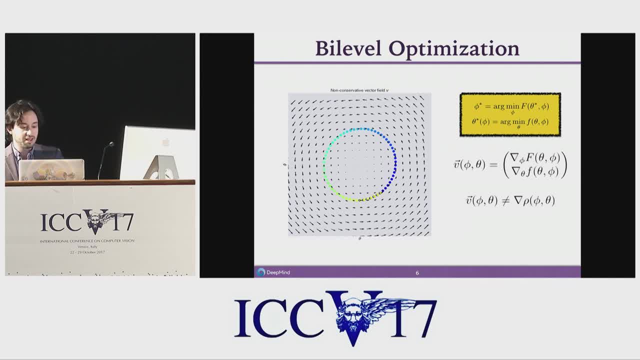 Deal: 0, 11, 6 Clock, Z p, 5, Z Z, 1, 6, Tra I, t, 3, 27, And most of the heuristics just come down to various ways of trying to solve this. There are sort of classic methods. for instance, there's one called Poliak averaging, where 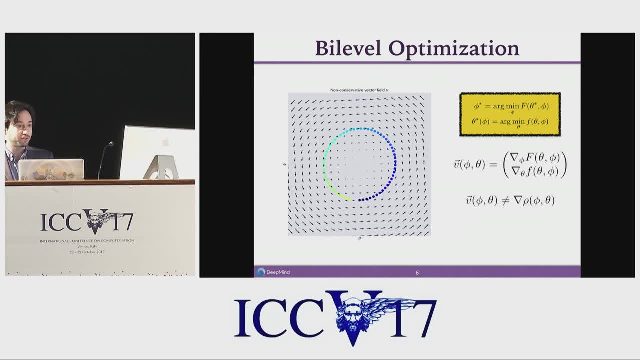 instead of doing a gradient descent step from the current value of your parameters, you do a gradient descent step from a moving average of your past parameters. That introduces sort of a drag term, which helps prevent these oscillations, even though it slows down learning somewhat. 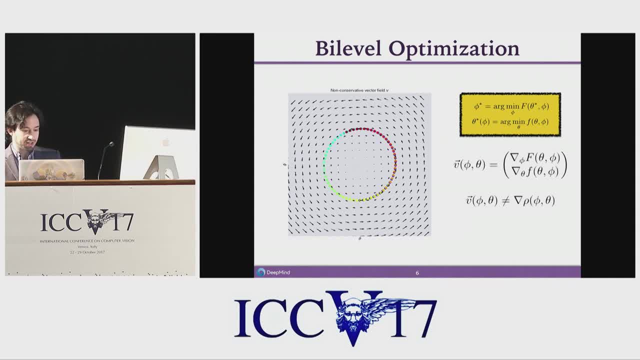 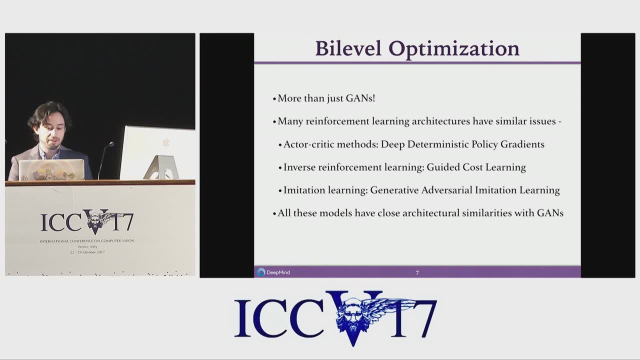 Now this, as I've said, is not just a problem with GANs. I'm going to go through a lot of the other optimization problems that share this problem. So in the world of reinforcement learning, you have a lot of actor-critic methods, such 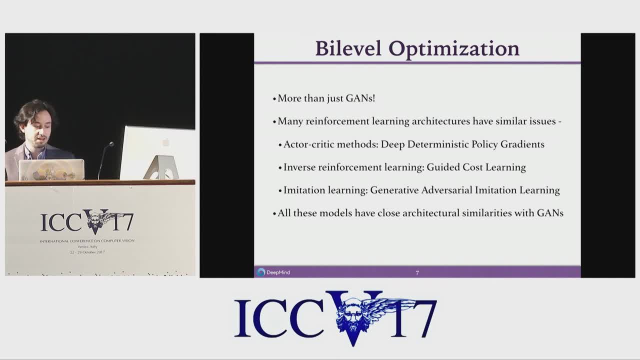 as deep deterministic policy gradients that suffer from these problems. In the world of inverse reinforcement learning, it turns out that an algorithm called guided cost learning is actually formally equivalent to GANs under certain settings, And there are many problems in imitation learning that are also naturally framed as an adversarial 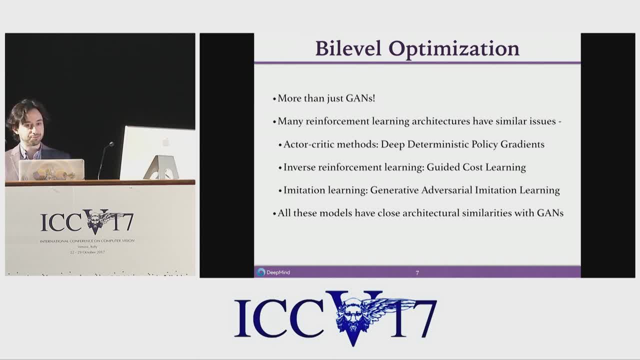 problem. So there are actual. there's been recent research actually combining generative adversarial models with imitation learning, And so these all have close architectural similarities And therefore the heuristics of GANs are very similar. They're very similar. 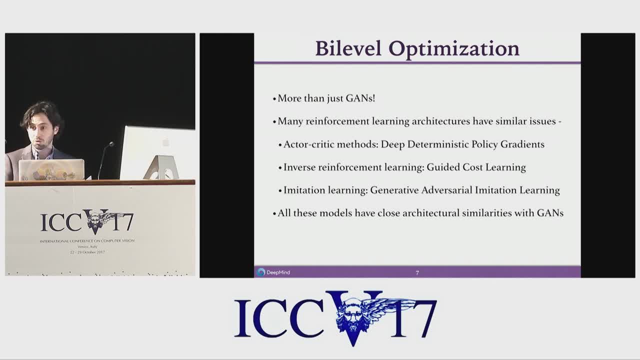 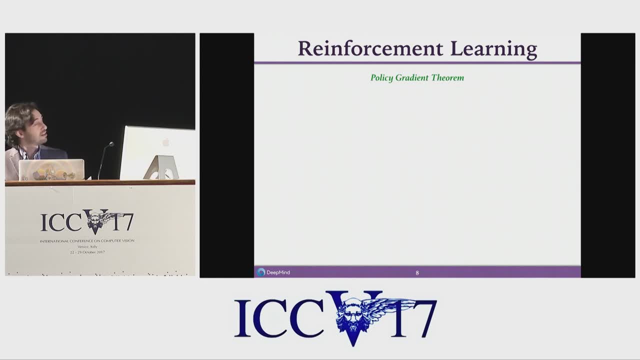 But the heuristics that we use for training them, we would hope should transfer between these models. So you've all heard a lot about GANs today, But a very, very quick overview of the problem of reinforcement: learning sort of reinforcement. 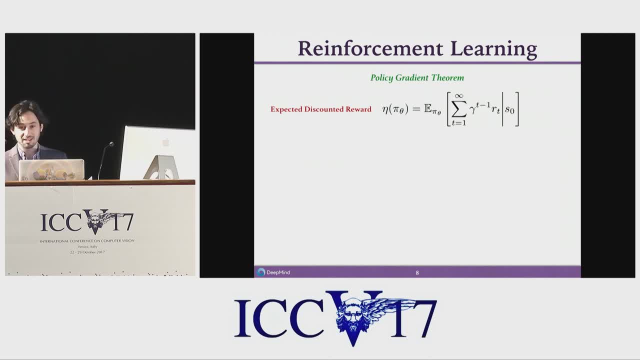 learning in one slide. the basic object of study is how to optimize the value of policies in a Markov decision process. So you have some kind of either one step or sequential game where you have a number of different states, denoted s a number of different actions that you can perform in. 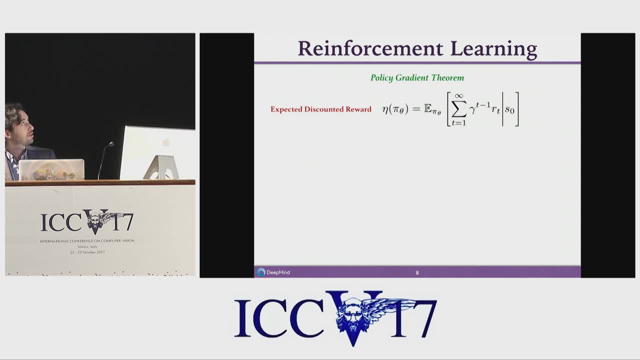 those states. You want to learn a policy, denoted pi, that for every possible state gives you a distribution over actions, And often that policy is a parameterized policy. It's something where you use some kind of function approximation. So we denote the parameters for that policy with theta. 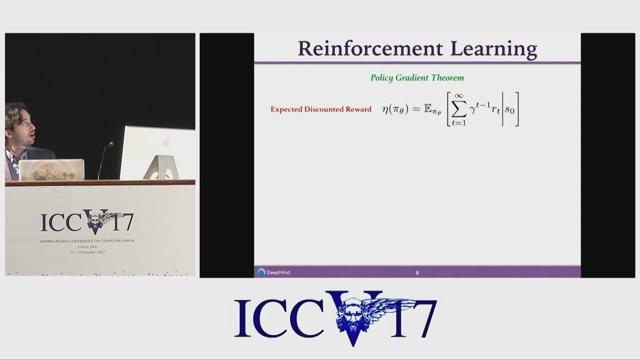 And with every action that you take you get some reward denoted r, And the goal is to maximize the discounted long-term reward of your policy. So you have this discount factor gamma that just tells you how much to value current reward over future reward. that just makes sure that your long-time horizon reward is bounded. 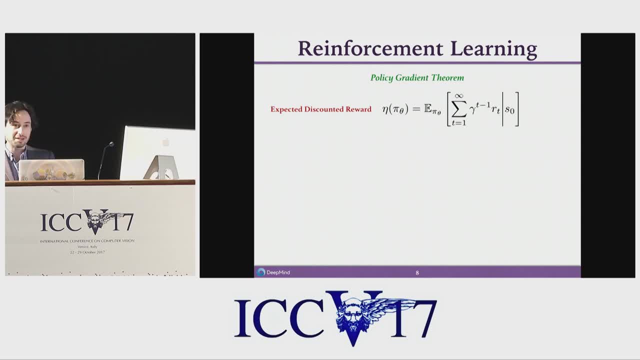 And the whole field of reinforcement learning basically comes down to different ways of optimizing this function: eta, this expected long-term reward. So one very common method that goes into methods like Q-learning is to learn a value function and implicitly learn the best policy by instead learning the expected long-term value of any 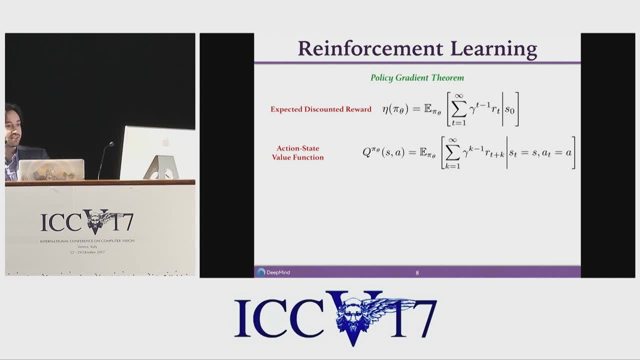 action in each state. So this Q function says, for any particular policy, If I'm currently in the state s and I take the action a, what is my discounted long-term expected reward for that particular state? And then the optimal policy is just to look over all of the different actions and take. 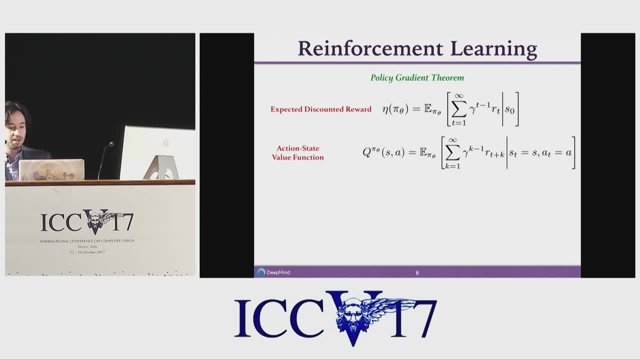 the one that gives me the highest expected reward, And this is a form of implicit policy learning. but you might also want to directly optimize your policy. So let's say you have a gradient descent, in which case you have to compute gradients of this expected reward, eta, with respect to the parameters of your policy. 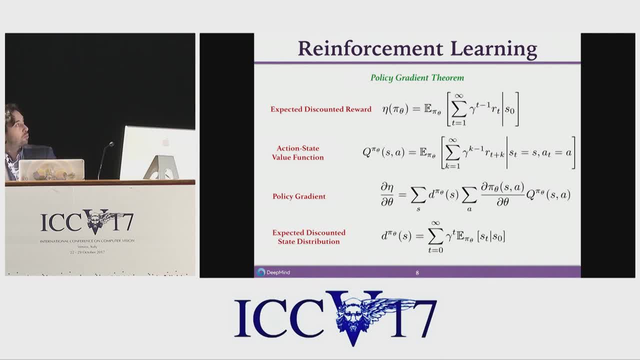 And so there's a classic result called the policy gradient theorem, which says your gradients of eta with respect to theta take this form, which is: it's the discounted expected product of the gradient of your policy times, the Q function. So if you actually knew the true Q function, this would be great because you could exactly. 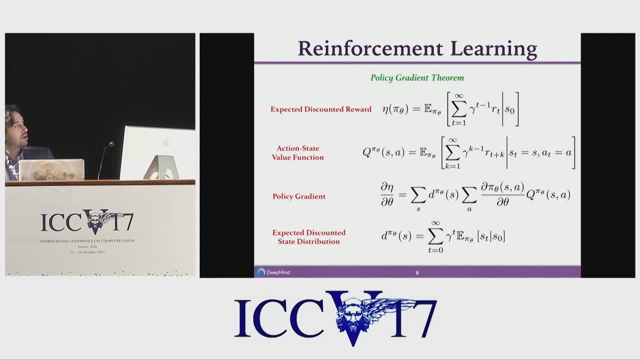 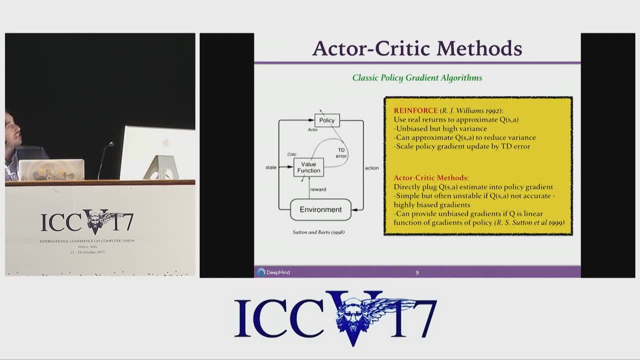 compute gradients. In general, you don't actually know the value of Q, so you now sort of have two unknowns that you have to learn. So architecturally, this kind of looks like this: You have this policy and a value function that you simultaneously want to learn, while 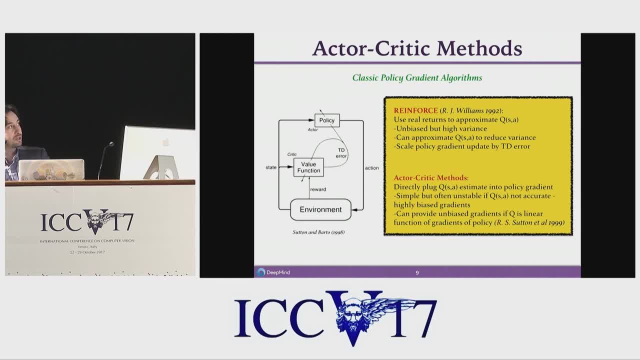 interacting with the environment and get error signals going between these models. One of the first dogmas of this model is that you can actually compute gradients. So if you actually knew the true Q function, this would be great because you could exactly compute gradients. 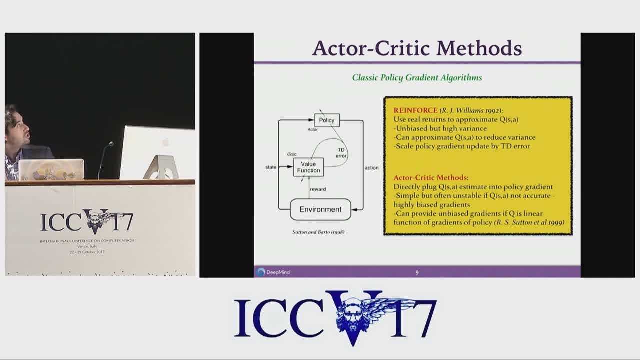 The other two algorithms for learning. this was the REINFORCE algorithm, which just uses returns from episodes. It just uses the observed rewards as an estimate for Q. but that's very, very noisy in general And these methods REINFORCE typically learns very slowly because even though it gives 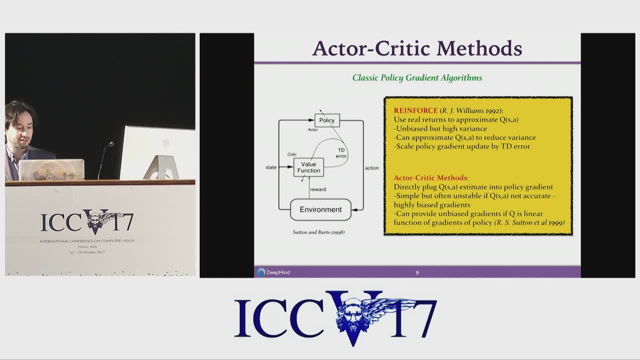 you unbiased gradients. it gives you very, very high-noise gradients, So it's slow to converge. The other idea, and the one that's more relevant for GANs, is actor critic methods, And there you use some kind of function approximation. 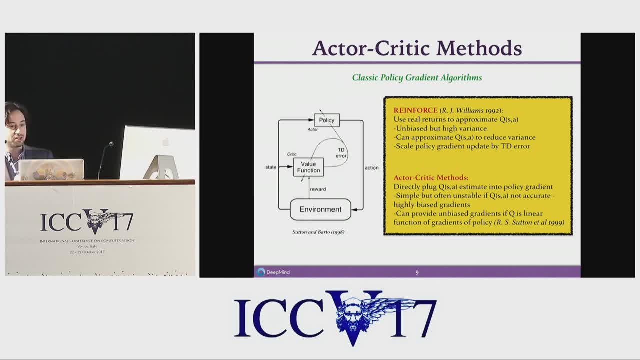 But this method is very, very slow, both to learn Q and learn the policy pi simultaneously. but if your Q estimate is very inaccurate, the gradients that you get will be highly biased and these models are sort of notorious for suffering from collapse during training, where they'll just fall onto degenerate solutions. 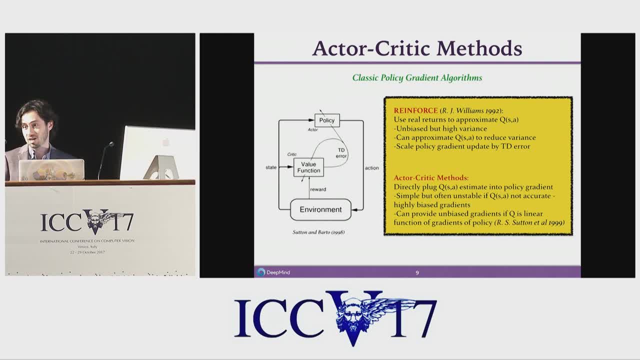 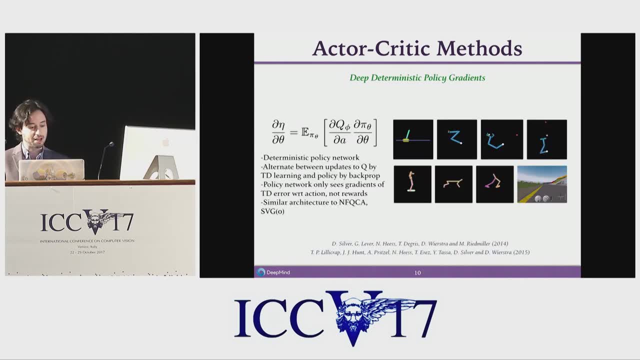 And very similar to the way that GANs are notorious for also falling into degenerate solutions if you're not very careful in training, And we can make that a very precise connection, as I'll describe. So despite these difficulties in training in recent years there have been a lot of practical. 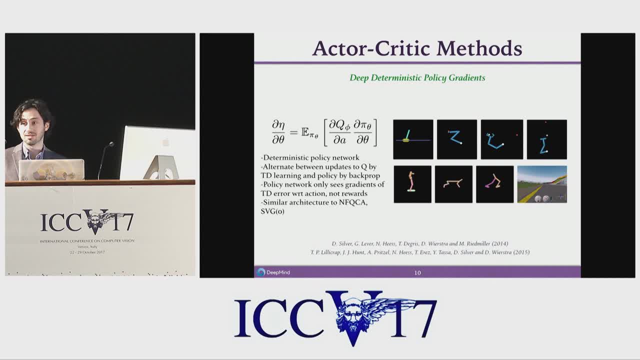 successes of these algorithms. One of the most prominent actor-critic methods to come around in the last few years is what's called deep deterministic policy gradients. So this is specifically where you're using a neural network to learn a deterministic, rather than stochastic, policy pi. 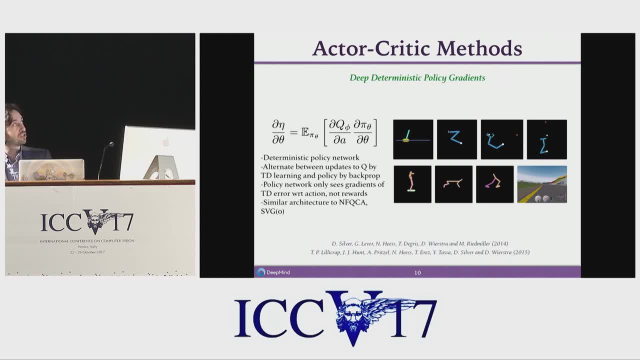 And this is useful in sort of robotics tasks like learning to grasp- Let's see Learning to walk. So here are some examples of many different types of simple walkers that can learn to move using this architecture. You can even use it to learn to play simple racing games and things like this. 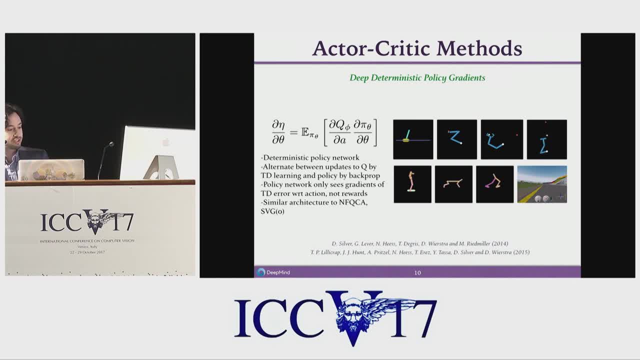 And the idea here is really the policy gradient just takes the form of back-propagating your error in your value function back through your Q function to your policy, And this has come up in a few different architectures. Take things called neurally fitted Q-learning with continuous actions or stochastic value. 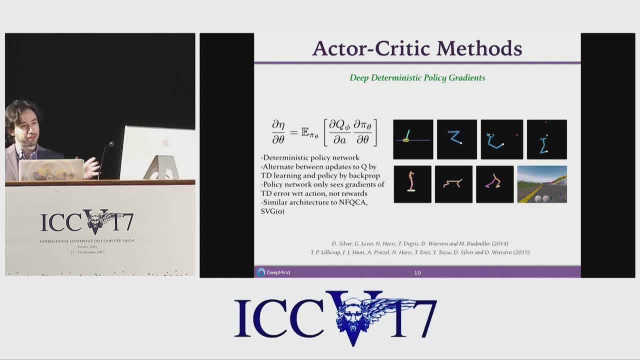 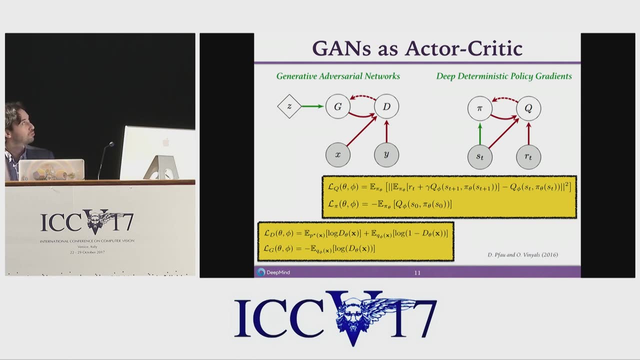 gradient zero. So they're all slight differences in the way these models are trained, but at the high level they all have this architecture And really the key idea- kind of connections between GANs and actor-critic- really just boils down to looking at this slide. 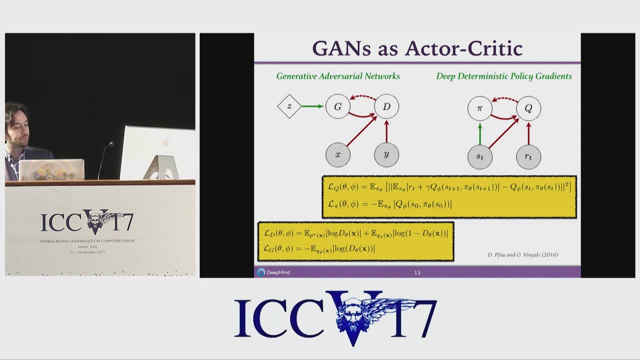 I'll just walk through what the symbols actually mean here So you can see here structurally, and even from the name actor-critic it's a little – you can sort of intuit what the connection is. A critic plays a role very similar to a discriminator. 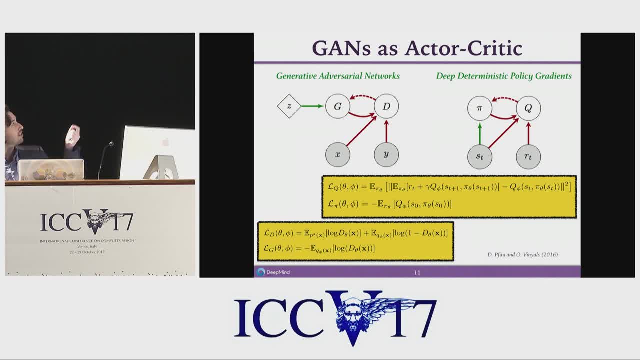 Here in the GAN setting, I'm using Y to denote this sort of signal of whether an image is true or false. while X is the generated – is a real image, Z is the noise that you pass to the generator And, in the case of deep deterministic policy gradients, both the policy and the Q function. 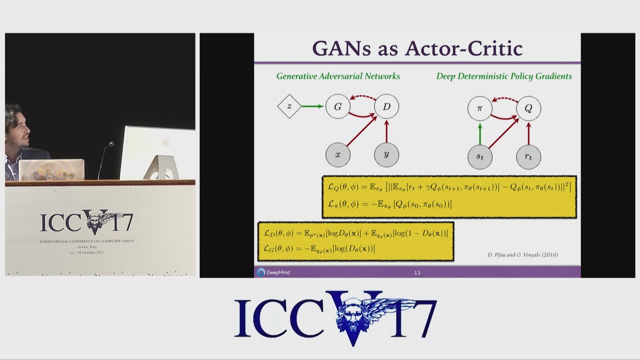 get access to the state, but only the critic Q gets access to the reward. So in both cases there's some privileged information that the discriminator or the critic has access to The reward, or the identity of an image is real or fake, And the – either the generator or the policy has to learn entirely from gradients of this. 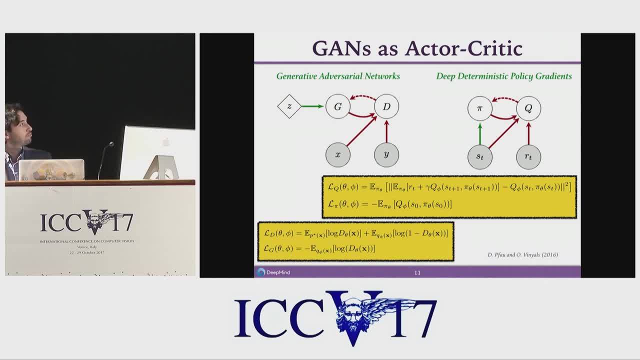 privileged information that are passed back to it. Obviously, there are also big differences between these architectures. Here on top, the actual loss function for the – for the Q function looks something like this: You're trying to minimize your difference in the prediction between the Q function plus. 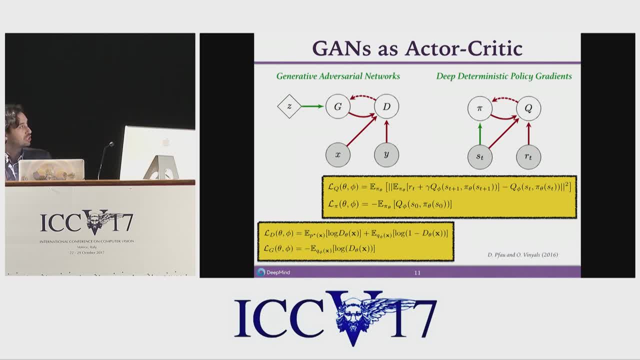 the reward at a future time step and the Q function at the current time step. So you're trying to guarantee that your critic – – obeys this self-consistency condition, that it predicts an accurate value function over time, while the discriminator has a slightly simpler job of just having to predict real. 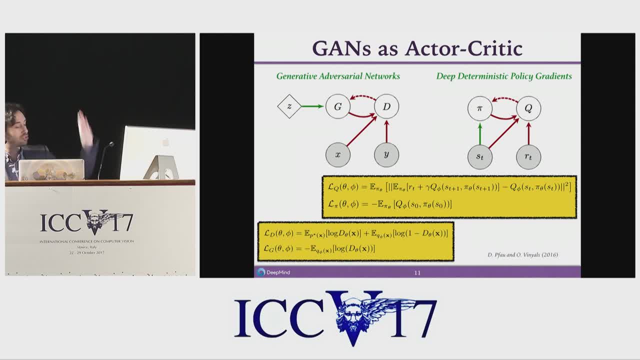 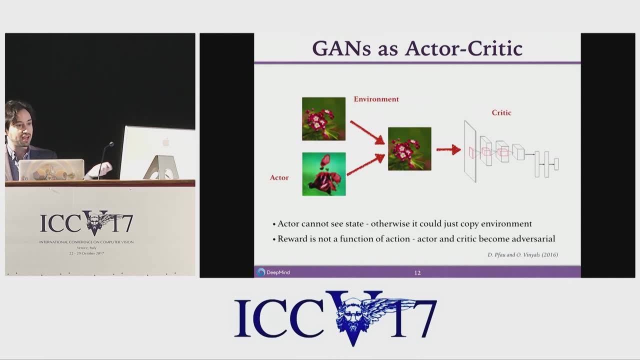 or false at a single time step, But structurally, hopefully, you get the intuition from the figure on top of exactly how these models are connected. So we can even make this a little more precise and describe a particular kind of Markov decision process that reduces down to GAN training. 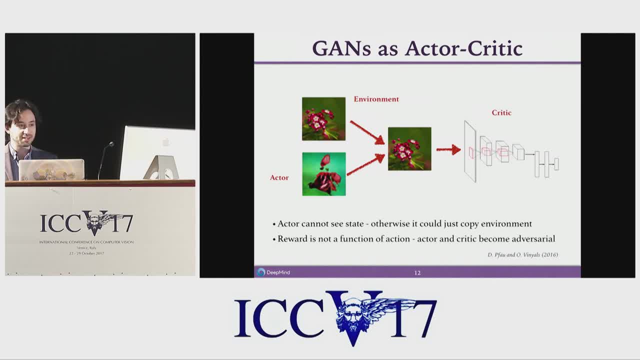 Usually the first question when I sort of mention these similarities is: well, aren't the actor and the critic – they're not really trying to do something adversarial? They seem to be trying to do something complementary. They're just learning different things. 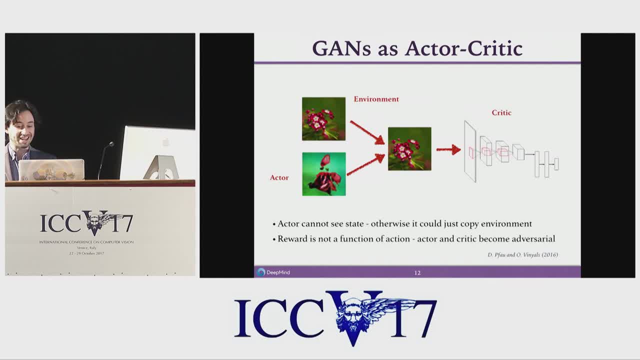 Whereas in GANs the discriminator and generator really are actually kind of fighting against one another And you can actually describe a sort of pathological game Where what should be two complementary models become adversarial. So you can imagine an environment where an actor can set every pixel in the environment. 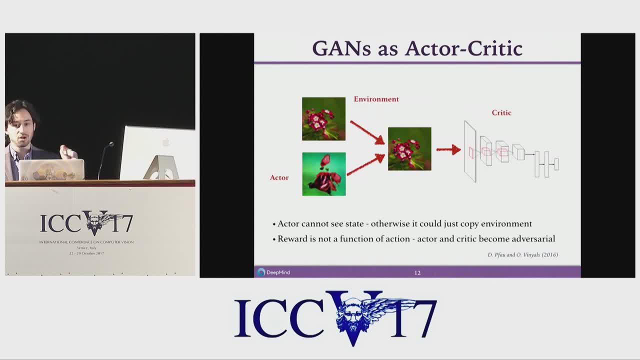 And then the environment decides randomly to either show what the generator has done, what the actor has done, or to just show a real image and give a reward of one if it's a real image and zero if it's generated. Now, this is an environment –. 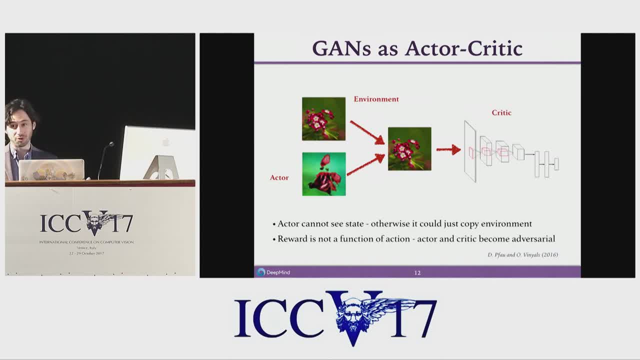 This is an environment where, no matter what the actor does, it can't actually influence the reward whatsoever. So it's actually kind of like a frustrating, like nihilistic kind of environment, because as hard as the actor tries, it's never actually going to get any better. 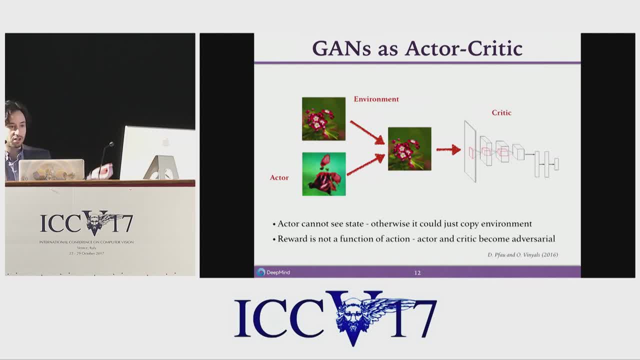 So the learning signal to the actor will encourage it to generate things that look more like real images, while the critic will learn that the actor isn't actually having any effect and down weight the value for those images. So what should be a complementary learning problem turns into an adversarial learning. 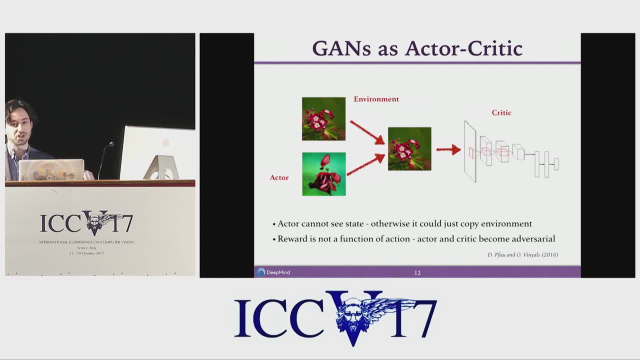 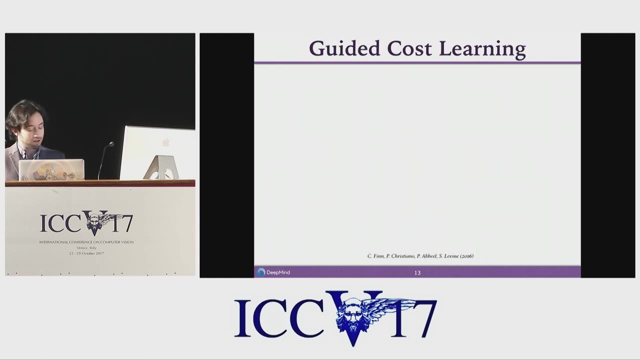 problem. So this is particularly kind of pathological from the point of view of reinforcement learning, but exactly becomes the problem in generative adversarial networks. So there are many other reinforcement learning algorithms that also have this bi-level or even tri-level structure, Some of which are not. 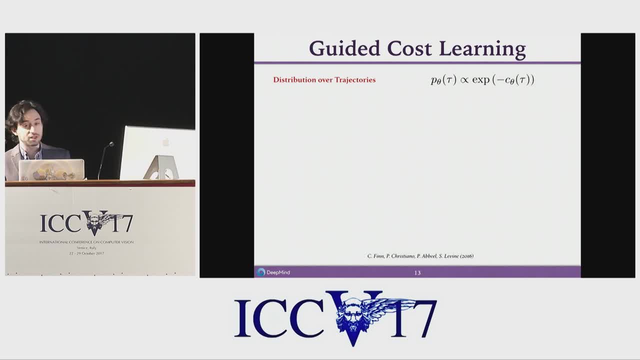 Some of which are connected to GANs in other ways. There's one called guided cost learning in the world of inverse reinforcement learning. So inverse reinforcement learning, as the name suggests, is a bit of a reverse of the task that most reinforcement learning is going for. 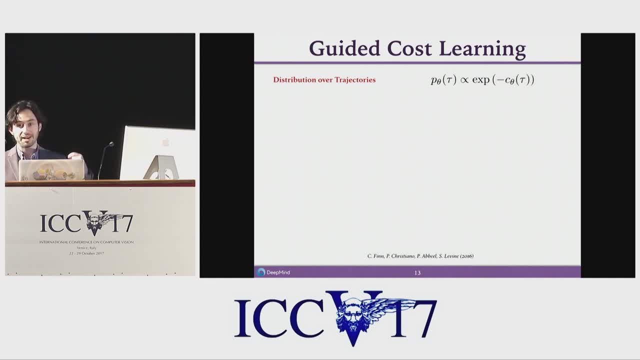 Rather than having a cost function and trying to learn a policy that optimizes the reward. you are given an example of expert trajectories and you're trying to learn a cost function such that those expert trajectories don't change. And those expert trajectories are what reinforcement learning would find. 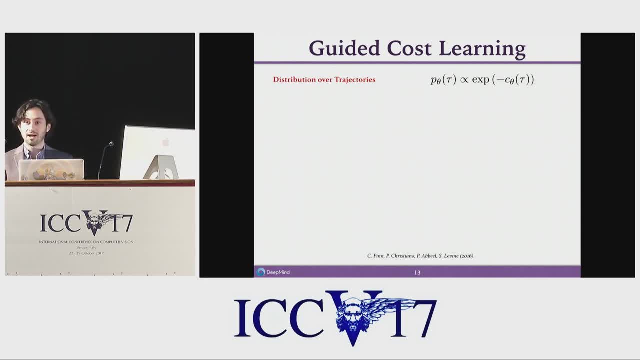 So again, this is useful in robotics if you have, say, an expert providing some control signal, manipulating a robot by hand, and then you want to generalize this small amount of expert data. So the idea here is that, given expert trajectories, you want to learn a policy such that you can. 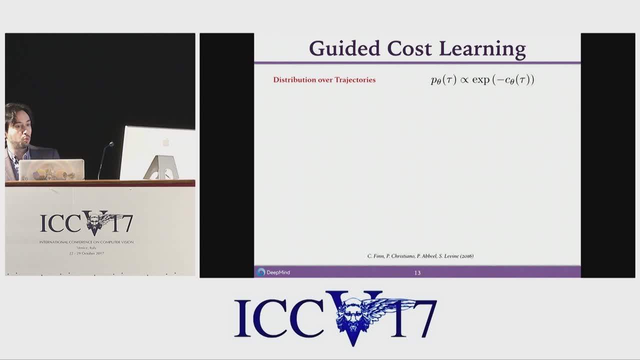 learn a maximum entropy distribution which assigns high probability to these trajectories. by having this maximum entropy term, that encourages some amount of diversity in the learned distribution And maximum entropy distributions. you generally don't know the normalizing function, so optimizing this directly isn't always feasible because this is an un-normalized probability distribution. 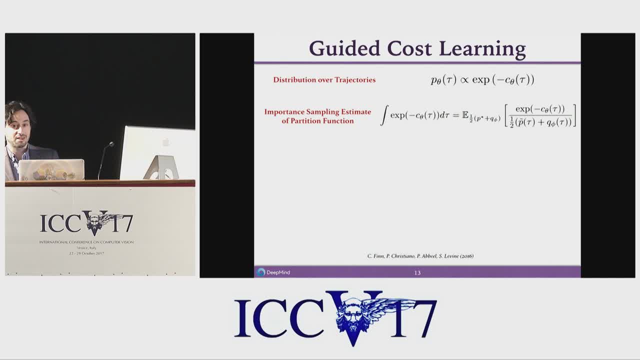 So you use importance sampling to estimate this loss. But importance sampling doesn't work very well if you don't have a very good sampling distribution. So you simultaneously want to learn a cost function and an importance sampling distribution that minimizes the variance of your estimates. 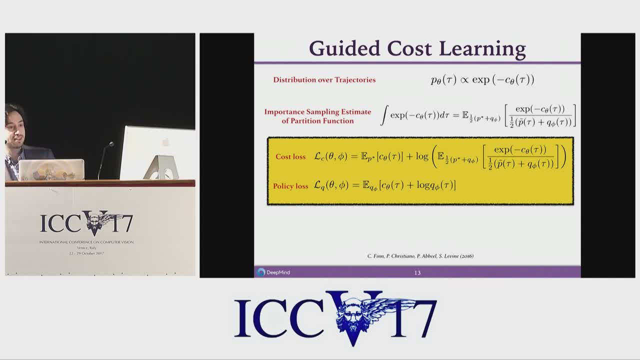 And you have two cost functions that look sort of like this and this term inside of the cost loss. 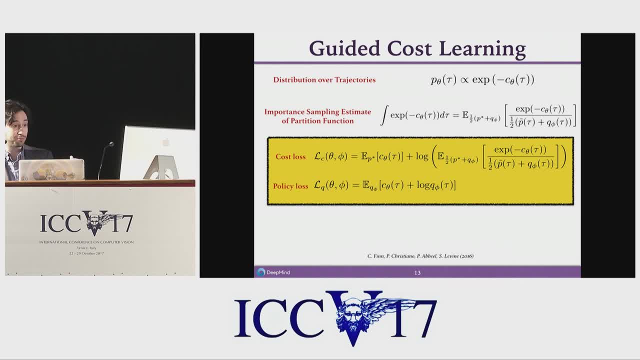 And this actually on the opposite side of the expectation, here, if you'll remember, looks a lot like the optimal discriminator in the case where you know the distribution And that turns out to be, mathematically, an exact correspondence. 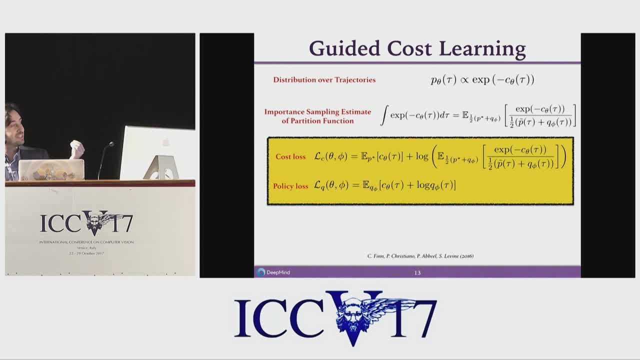 So if you actually know the density of your data distribution and the density of your sampling distribution, then the sampling distribution becomes exactly equivalent to a generator in a GAN and guided cost learning becomes. 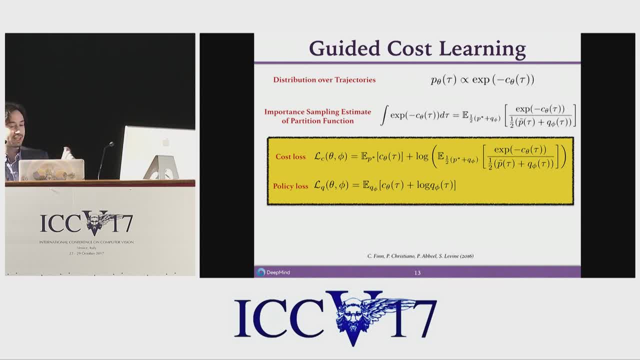 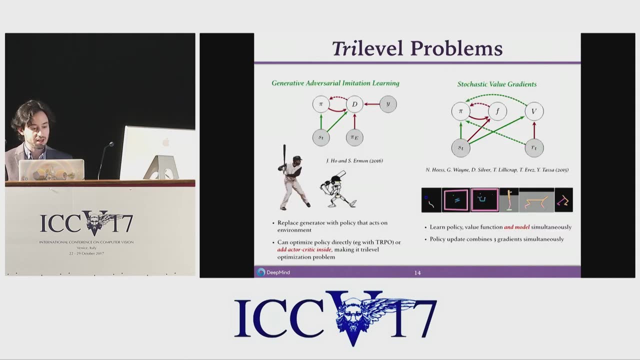 equivalent to learning a GAN, where you know the true density. Now, of course, the real motivation behind GANs is that you don't always know the true density of your generative model, but it is an interesting formal connection. And then there are even more complicated problems. 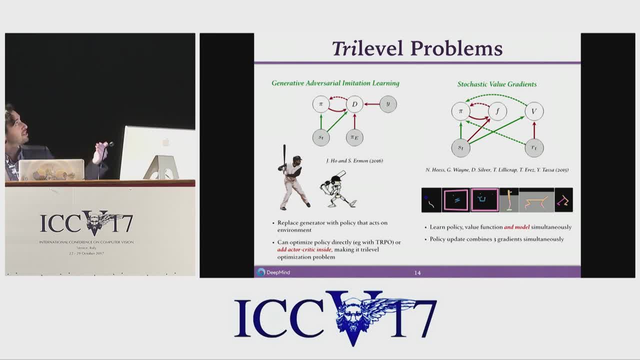 that are really tri-level problems, such as generative, adversarial imitation learning, which is similar, which sort of skips the step of learning a cost function in imitation learning and tries to learn a policy directly. So you can take an actor critic method and use that to try to learn a policy and then have a discriminator that tries to discriminate. 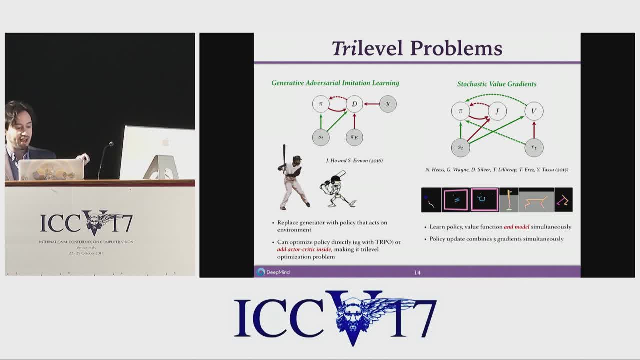 generated and expert trajectories, And so this becomes a problem that we're trying to solve. There's a problem of optimizing three models simultaneously, and then there are extensions to actor critic that also include a model on top of a policy and a value function. We're 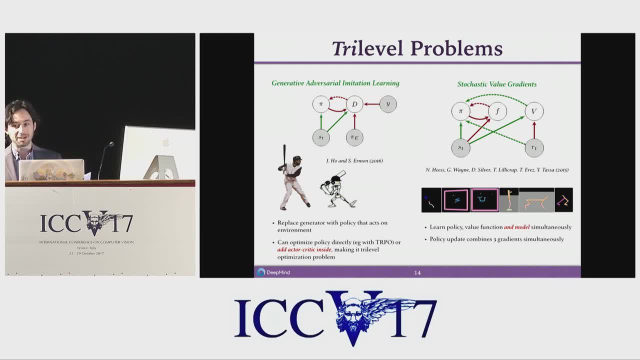 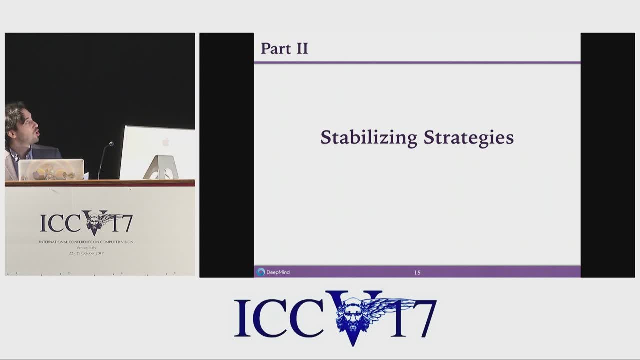 actually combining three different gradients together, so these become very, very complicated problems. So this has taken a little longer to go through than I'd hoped. but I want to talk at least about go through some of these different stabilizing strategies used in both communities, but I'll talk about them later. 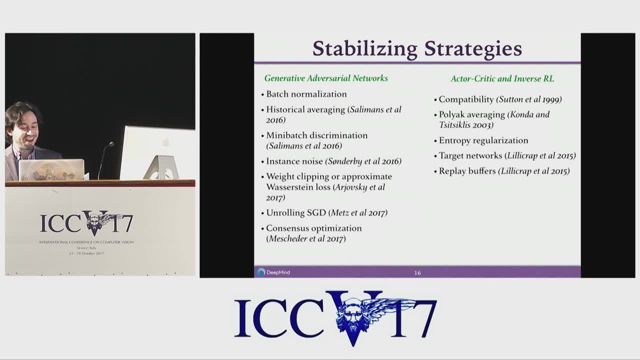 But I'll just sort of quickly run through these, because this is: you know, there's been such a huge explosion of work in optimizing GANs in the last few years that this is only really a partial list of all of the tricks and tips that people use. And actor critic. 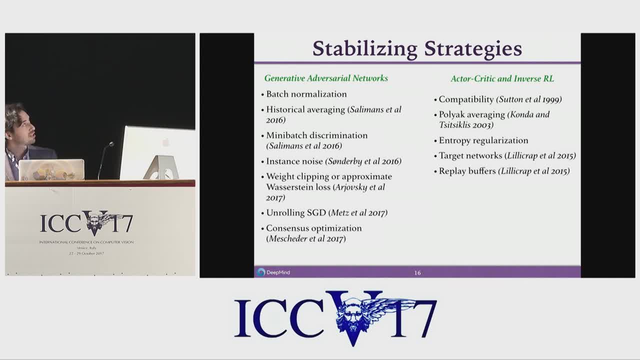 methods have been around for a long time but has been a somewhat smaller community, but I think still has some useful ideas to share. So, for instance, this polyac averaging that I mentioned at the start, where you introduce a drag term in your optimization. Okay, 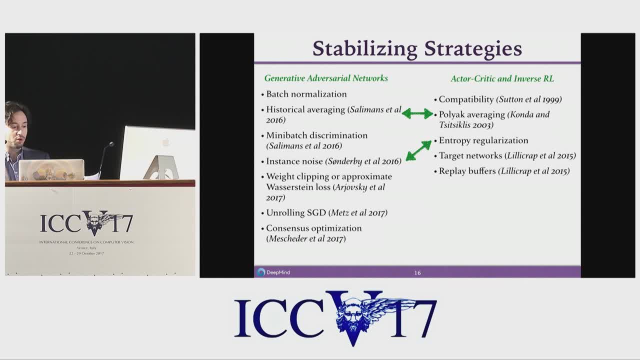 Okay. It's very similar to the historical averaging idea that Tim Solomons and others at OpenAI came up with in their techniques for optimizing GANs papers, The idea of instance noise, where you add noise both to the generated and real data sets to sort of help expand the support. 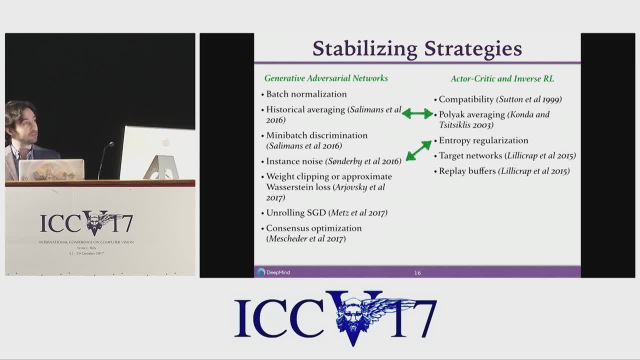 of the distribution of your generator is very similar in principle to the idea of entropy regularization in reinforcement learning. Okay, Where you make your policy sort of higher entropy than learning would suggest to encourage exploration. Otherwise it can just concentrate down too much on bad solutions. Some ideas: 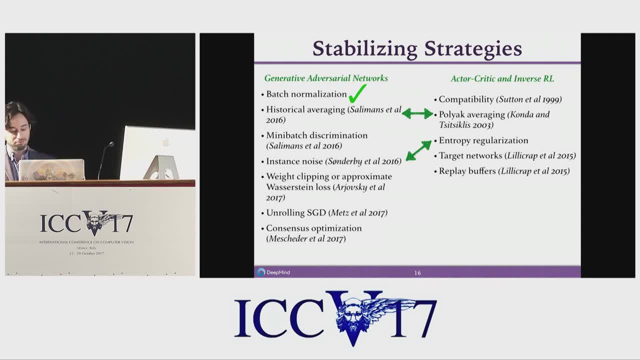 like batch normalization, are just good. Everybody should use them in any deep learning problem that you're using. Other ideas don't seem to transfer between the two communities. So, for instance, weight clipping as used in Wasserstein GANs- Okay In our experience haven't really helped in actor critic methods. The use of replay buffers. 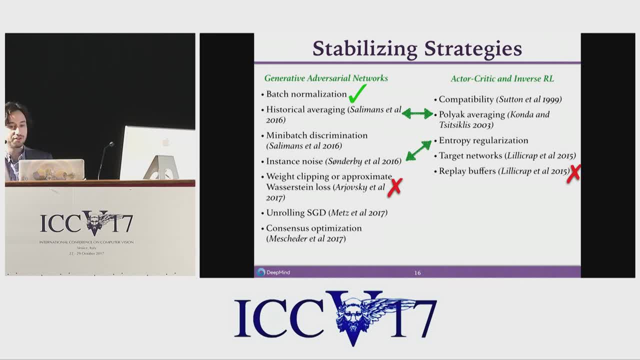 where you retrain with old data which help improve the stability of a lot of RL algorithms, don't seem to help at all with GANs. Some of these ideas for structural reasons can't transfer, but there are a lot of ideas where nobody in one community that, to the best of 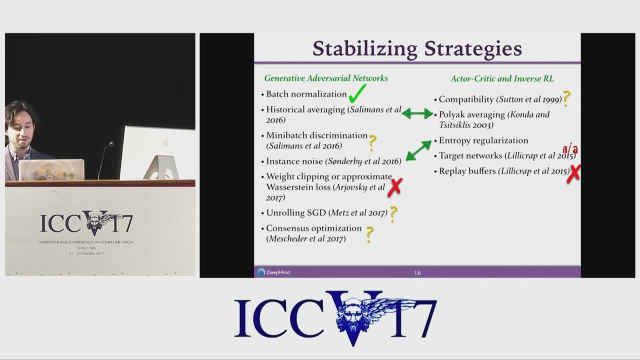 my knowledge has taken these ideas and tried them out in other areas. So I think getting people talking to each other and working together to sort of take the broader perspective on these problems and solving in a high level way is something we should pursue. And just one particular heuristic that can sort of work for all bi-level 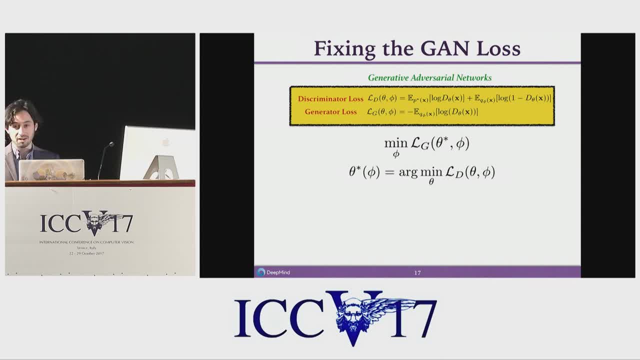 problems that I'll go through very quickly is this work on unrolling optimization, which was a paper We had at iClear this year, which is a sort of simple to implement idea for stabilizing the scan loss. So just once again, this is the optimization problem we're trying to solve. 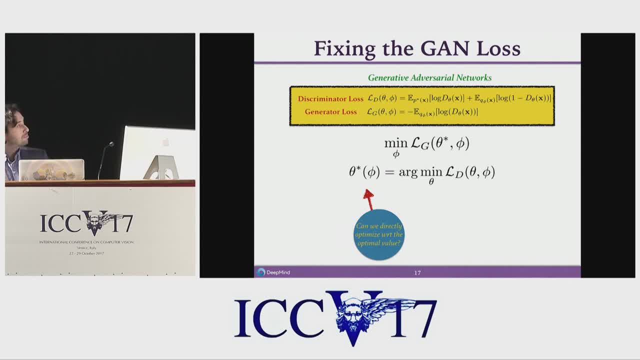 and ideally, we'd really like to be able to directly optimize with respect to this optimal value function, rather than optimizing from where the discriminator is at the current time step. We'd like to optimize with respect to the optimal discriminator, So the idea behind unrolled optimization is just to approximate this with a few steps of SGD. 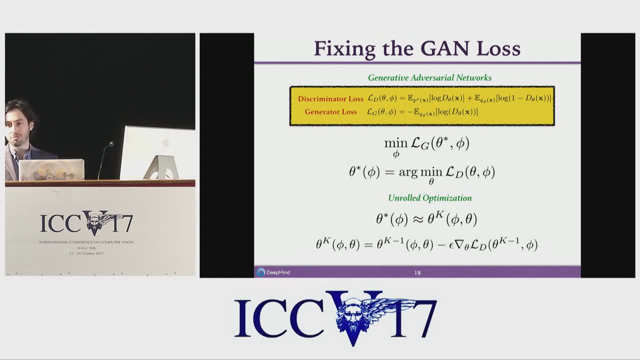 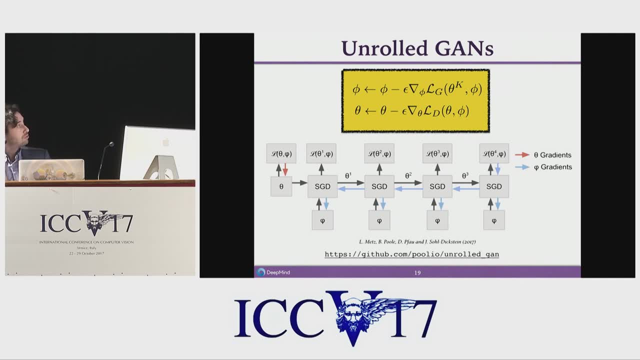 So this allows one model to look ahead into the future, into where the other model is going to be, and optimize with respect to that. So the sort of computational graph of this algorithm looks a bit like this: On the forward pass you run several steps of SGD, because each of these SGDs are not the same as the. 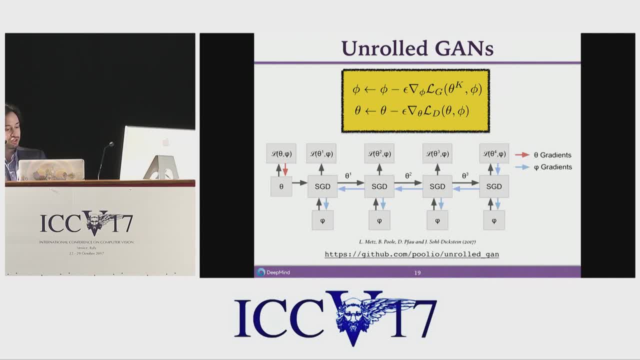 SGD boxes contains a gradient within it. When you actually do the backwards pass to optimize your loss for your generator, you're actually computing Hessian vector products, So this is actually a second order method. You're using information about the curvature of the value function between the generator and the discriminator to optimize this And 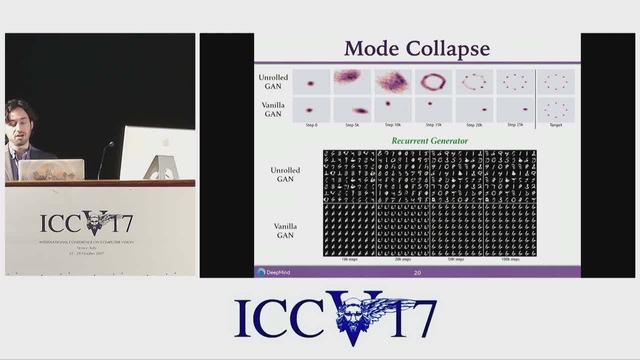 this helps fix problems like the sort of rock paper scissors problem or the sort of spiraling, endlessly spiraling problem that I gave at the end of the presentation. So this is a great example of how you can do this. So here's an example up top of trying to learn a generative model that has many different. 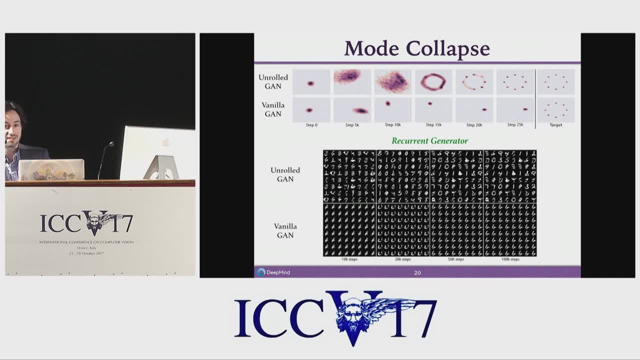 modes to it. If you just alternate between gradient ascent for a generator and a discriminator, it will just sort of circle endlessly, because the generator will just concentrate down on one mode and the discriminator will learn to classify that particular mode, pushing the generator off to the next mode. With unrolled optimization, the generator can look ahead. 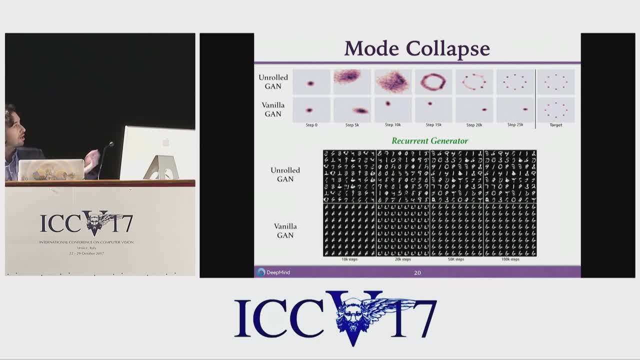 and spread its mass out On a more challenging problem. this is a GAN trained on MNIST, where the generator, instead of being a feed-forward network, is a recurrent network, And this is the type of optimization where things often fail, But using this unrolling optimization instead of collapsing down onto 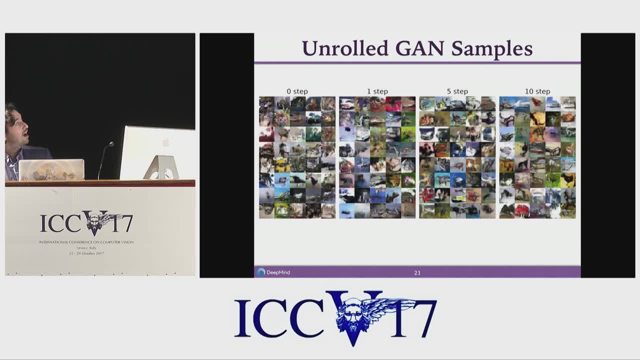 a single sample, we get much more high diversity samples. You can look at these samples and try to squint and see which one you like more. This is your own own example of how you can use different numbers of steps of unrolling. I think the 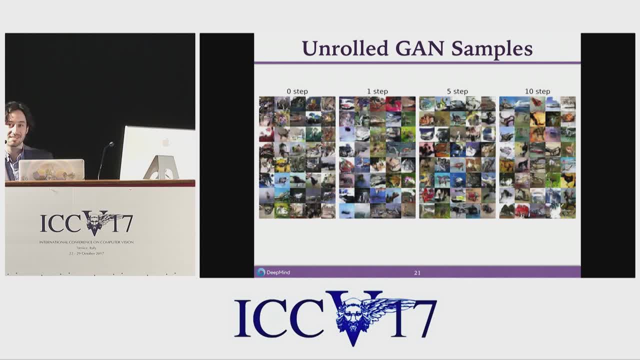 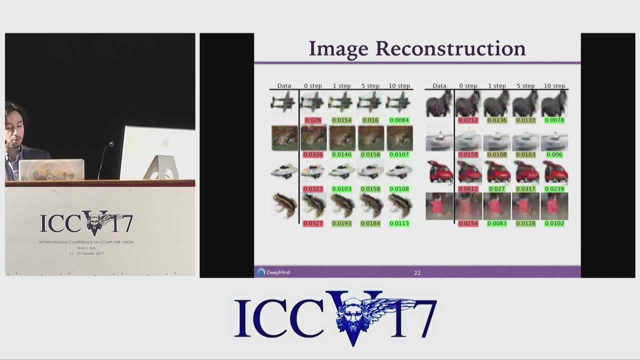 samples with the most steps look the best. but as with everything with GANs, it's a fairly subjective judgment call And to try to quantify this a little bit more, we tried to reconstruct out-of-sample images just by directly finding the optimal code in the in-generator space and found that the 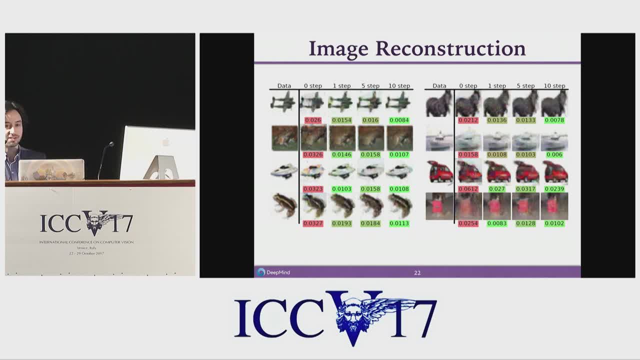 models tried to match the sample. So we found that the models tried to match the sample trained with more steps of unrolling we're able to find reconstructions that optimize this more accurately. I'm running out of time a little bit and want to leave a little bit. 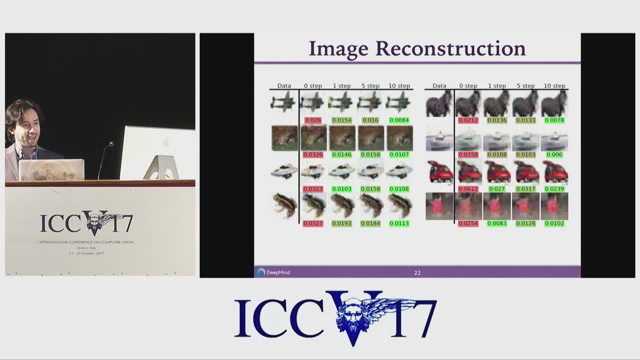 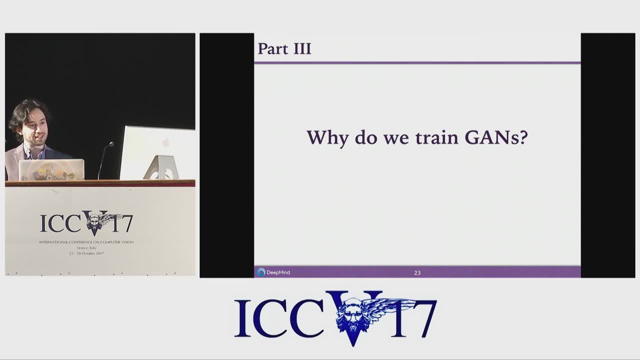 of time for questions, but I just want to sort of end on a bit of a more sort of philosophical note, sort of step back and ask: like why are we specifically thinking about GANs? Like how broad of a perspective should we take? What are the right tools for us to use? Because 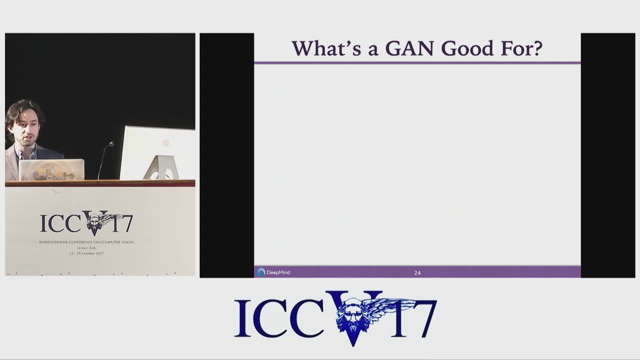 there are a lot of difficulties when we try to do generative models in the GAN framework, As this talk and other talks have attested to. like stability is an issue. By framing the problem as a minimax problem, you don't always have a good way of evaluating training. 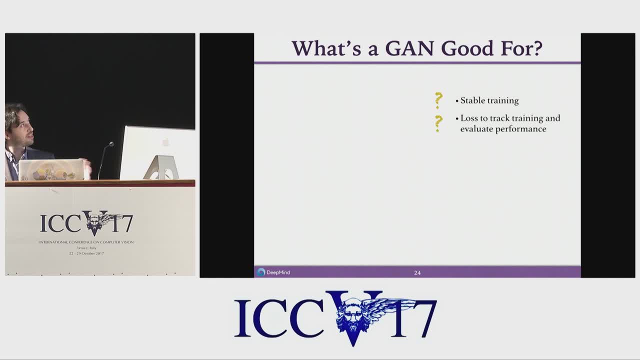 progress, though there has been some work like Wasserstein GANs that address this somewhat. Inference: you have to sort of add things like adversarially learned inference. You have to put inference on top. after the fact, It's not really natural to put inference into. 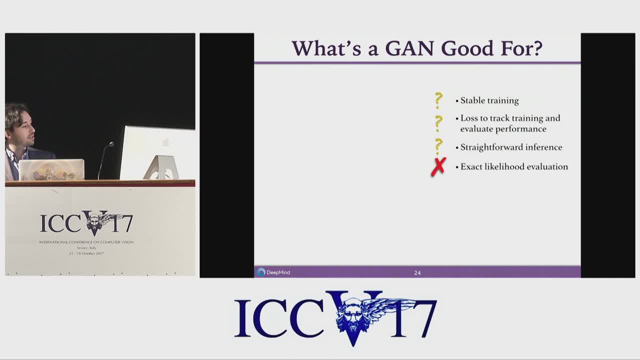 this framework. The motivating idea behind GANs is that you give up on exact likelihood inference, with the tradeoff being that you can try a wider range of generative models. You would hope that you would at least be able to do accurate density estimation, but 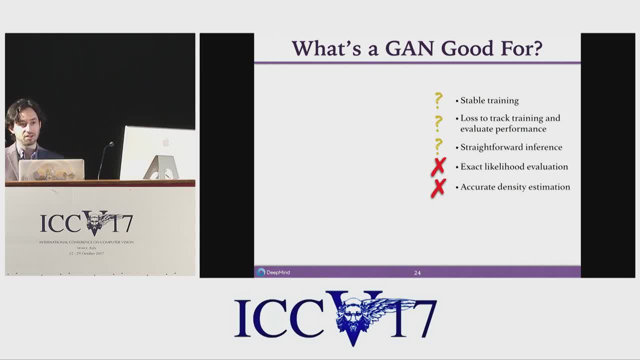 as Sanjeev Arora attested to, you don't really have good guarantees there. What we gain in exchange for this is this interpretable latent state where you can sort of do nice walks through parameter space, And really the biggest one, the one that 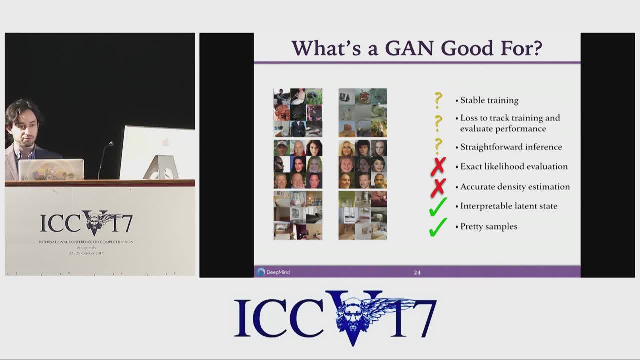 I think got people really excited about GANs is that you have these really beautiful, very sharp, clear samples. Like you know, comparing the real images on the left to the generated images on the right, you almost can't tell them apart. 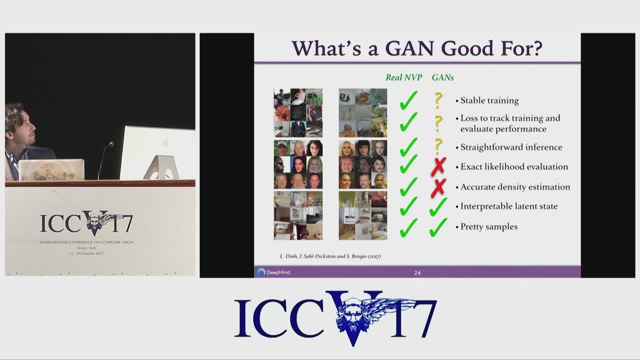 Except I've pulled a little bit of a bait-and-switch here. These are actually samples from a model called Real Non-Volume Preserving Flows. This was a recent work at ICLR, where you have a fully invertible generative model so you can do things like exactly calculate the likelihood. 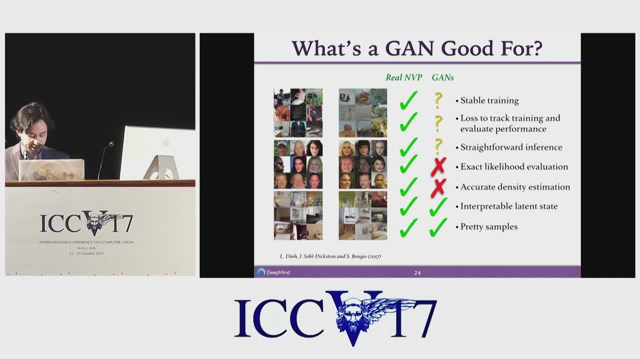 and just directly train through maximum likelihood. So when GANs first appeared on the scenes they were really sort of the first generative model that had very, very sharp, really sharp, realistic-looking samples, But in the last few years more maximum likelihood-based. 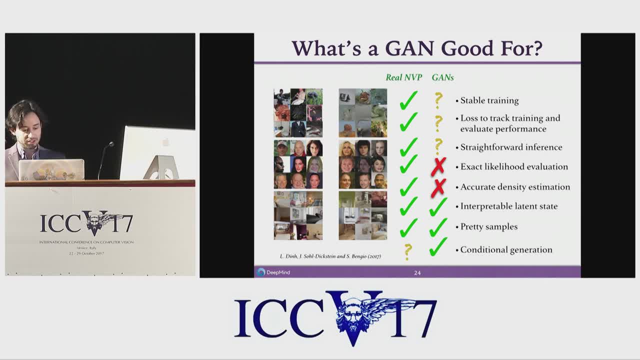 approaches I think have caught up. So I don't want to be too hard on GANs and say the one thing: where I think they still really excel is in conditional generation, things like picks-to-picks and super resolution, as we've seen in some of the talks today. 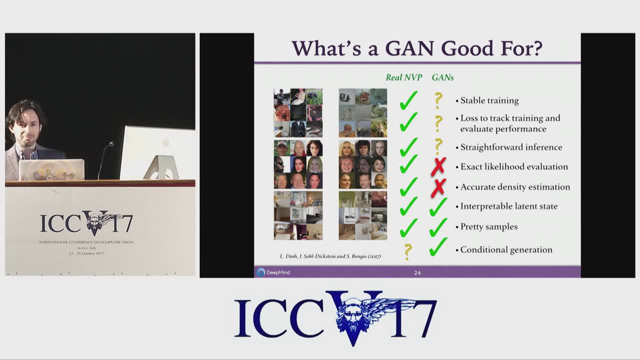 No other kinds of models have really caught up in terms of performance. But I just want to sort of say, as sort of message to the crowd, I want you all to sort of think carefully. if you're interested in GANs, really ask yourself what's the problem that you're trying to solve, Because if you're, 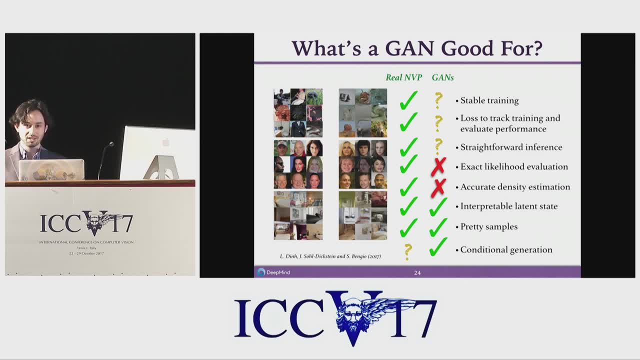 primarily interested in just a sort of standard generative model. there's lots of progress being made in the maximum likelihood framework. But if you're more broadly interested in problems, in adversarial learning and even beyond that in bi-level problems like the kinds that, 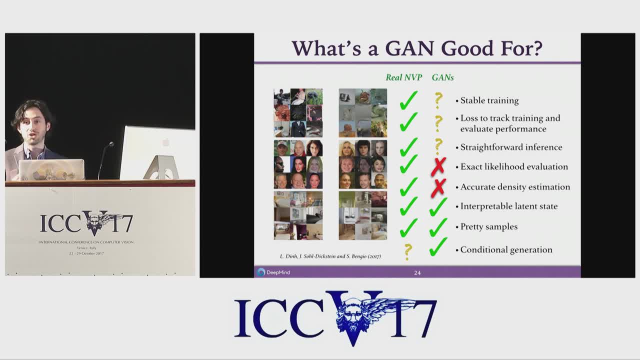 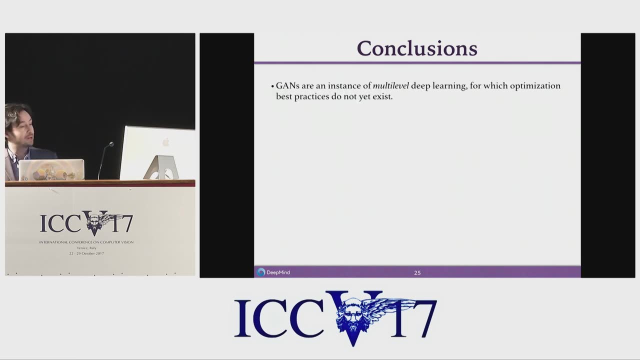 crop up in in reinforcement learning. I think there are huge opportunities for finding connections between these areas and, by building better training, really expanding the frontier of the kinds of models we can train. So just to sort of wrap up, give a quick summary: GANs are just one instance of this. more general, 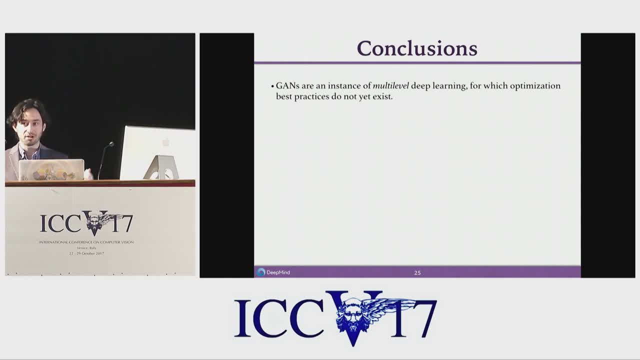 framework of multi-level optimization In deep learning, we're still sort of as a community trying to find best practices. This comes up all the time in actor-critic methods and inverse reinforcement learning problems and many other problems that are naturally framed as adversarial problems. 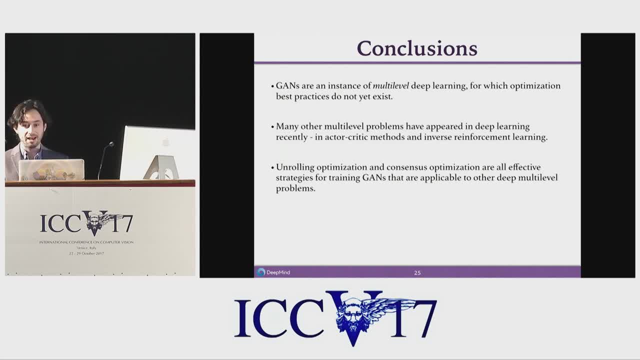 Unrolling optimization is one heuristic that has the potential to transfer between these problems. There's another nice one that I didn't have time to talk about, called consensus optimization. It's a recent paper at NIPS And, again, if your goal is to just train a, 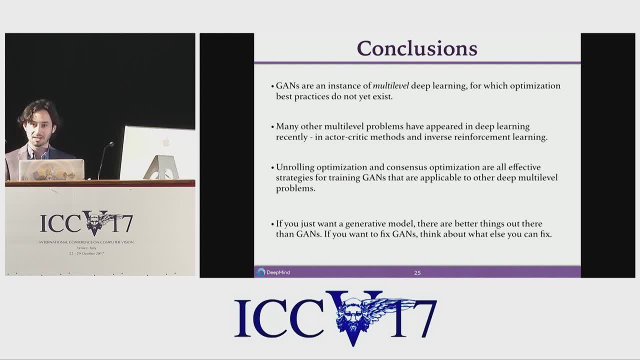 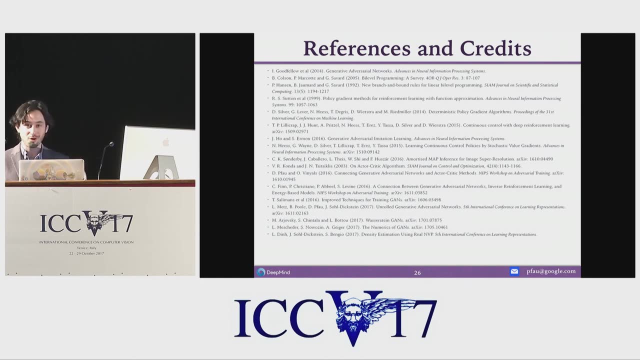 generative model, maybe think more broadly about what the techniques are out there. But if you So, if you do want to fix GANs, say, you know, try to do it in a way that fixes other things too. And so with that I'll say I obviously went through more than I can talk about, or more.